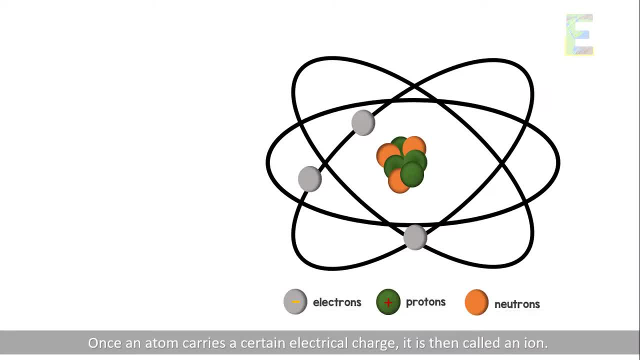 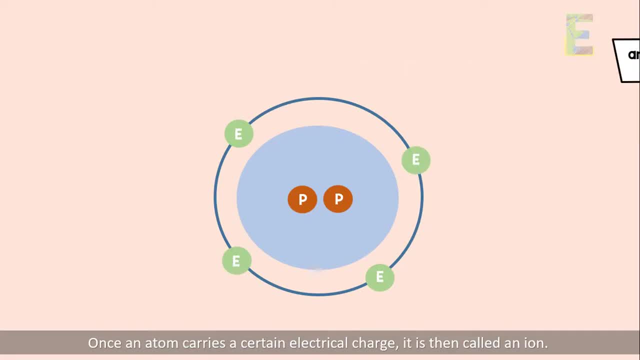 atom can gain or lose an electron. Once an atom carries a certain electrical charge, it is then called an electron, An ion. An atom that loses electrons creates itself as a positively charged ion called cation. Well, if an atom gains an electron, it becomes a negatively charged ion. That 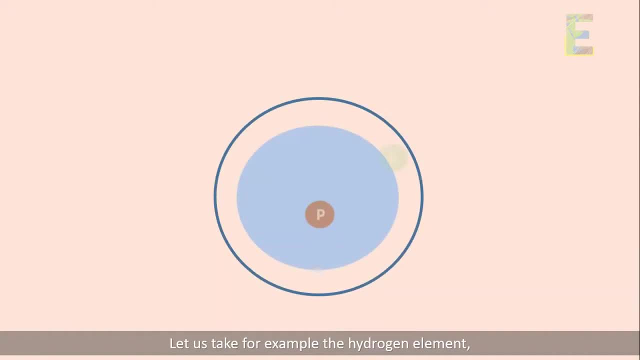 is called an ion. Let us take, for example, the hydrogen element. It is generally a neutral atom with one electron and one proton. Remember that the number of protons is fixed or unchanging. So how are we going to make this an anion or cation? 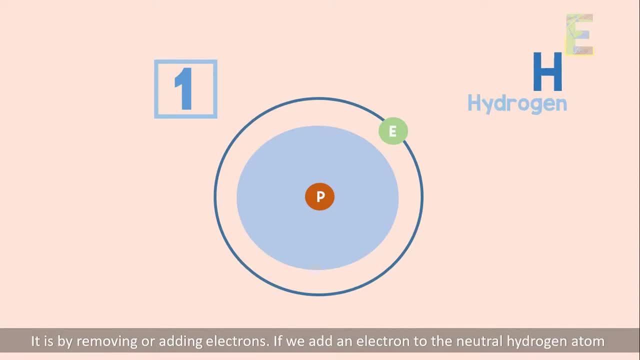 It is by removing or adding electrons. If we add an electron to the neutral hydrogen atom, it will then have two electrons and one proton. Then net charge is negative. Thus it is an anion. But if we remove the subatomic electron in a neutral hydrogen atom, 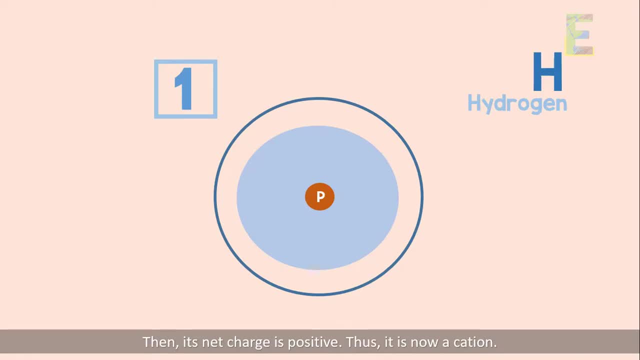 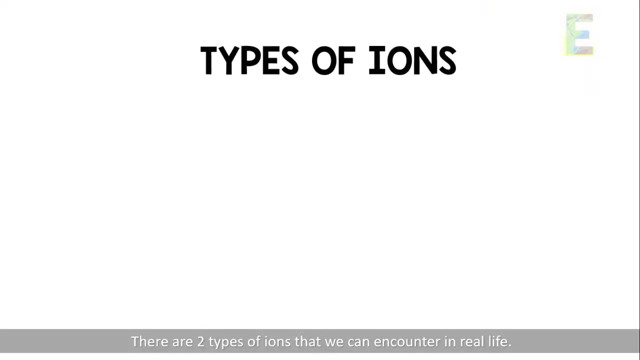 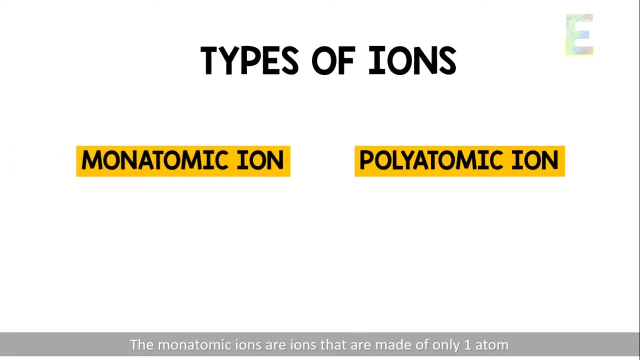 it will only have one proton, without electrons, Then its net charge is positive. Thus it is now a cation: Anion, Anion, Anion, Anion, Anion, Anion, Anion. The thieves forward. pictureATOM. economically, 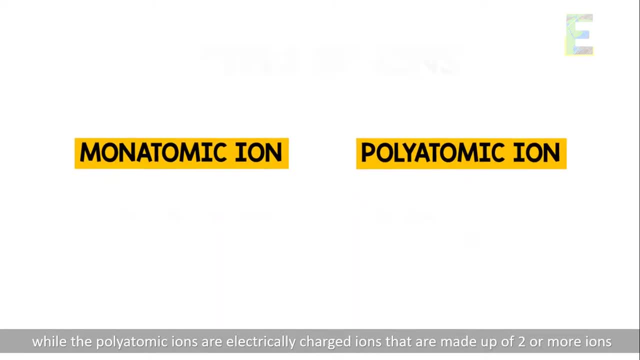 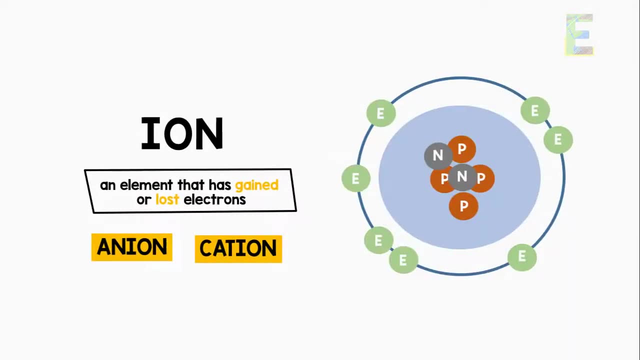 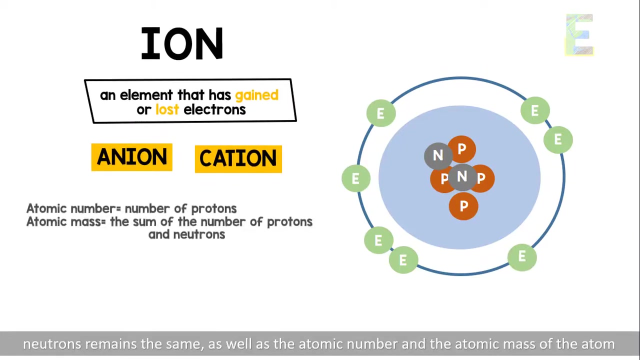 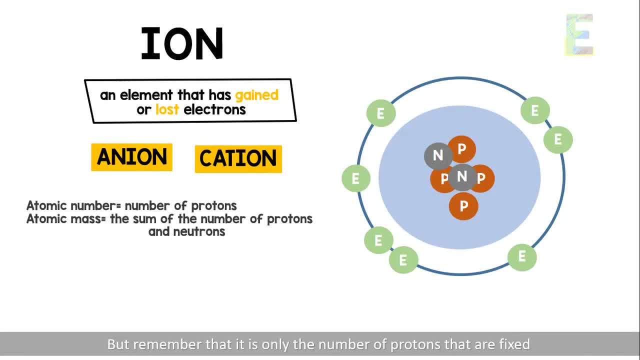 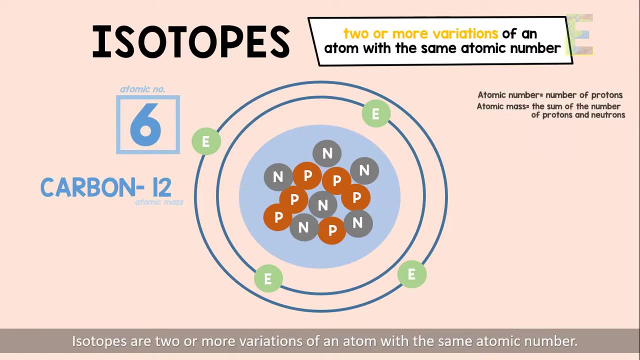 and the atomic mass of the atom, but remember that it is only the number of protons that are fixed. so how about we vary the number of neutrons instead of elections in an atom? this is the concept of what we call isotopes. isotopes are two or more variations of an atom with the same atomic number. however, isotopes 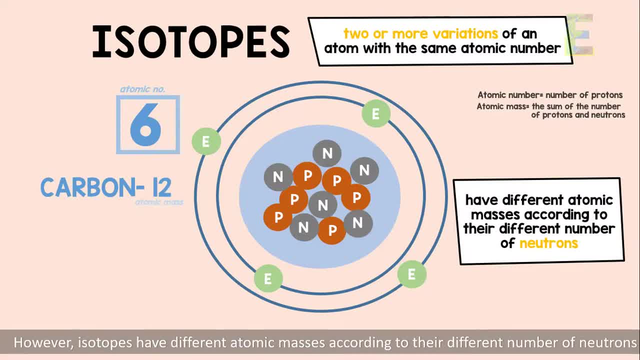 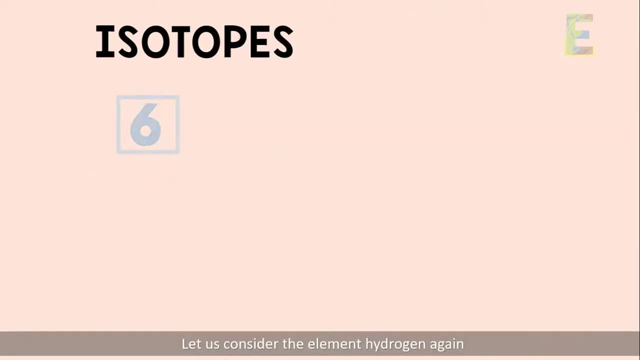 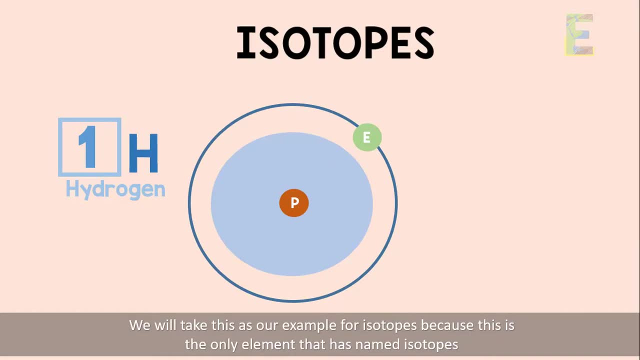 have different atomic masses according to their different number of neutrons. this means that isotopes do not change the element, the number of protons and the number of electrons. let us consider the element hydrogen again. we will take this as our example for isotopes, because this is the element that has named.